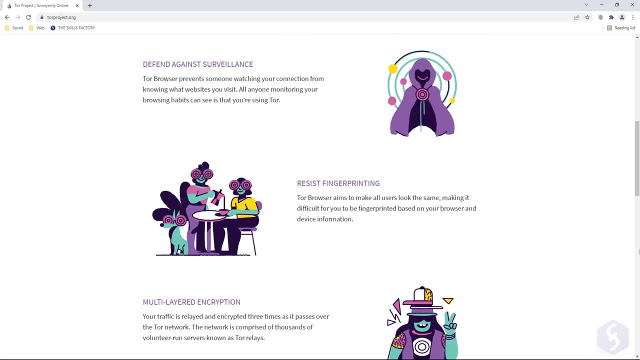 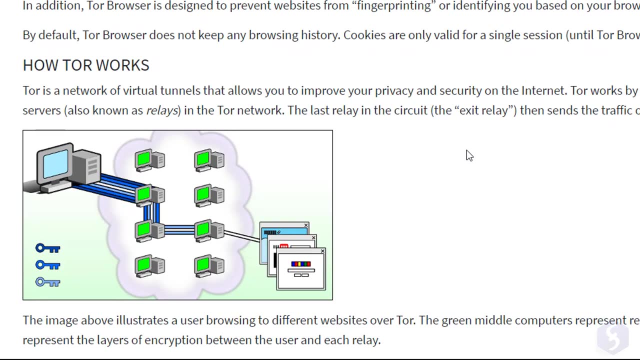 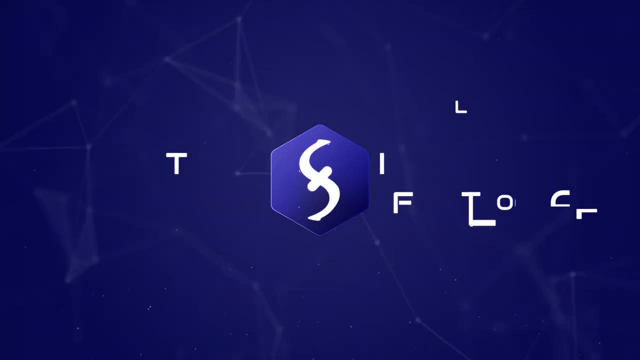 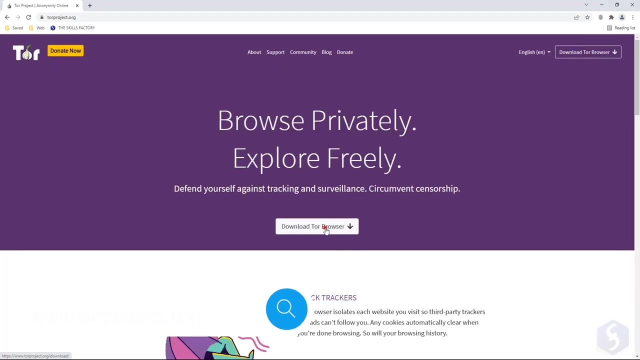 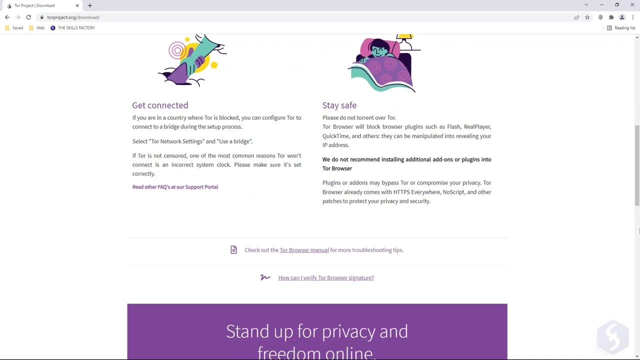 Hello, welcome to this new tutorial. Let's discover how to use Tor Browser, the best one to surf the internet with the maximum protection over your data, thanks to its network protocol based on Onion Routing. To download Tor Browser, go to torprojectorg and click on Download. This is completely free and it is available for Windows, Mac, Linux and also Android. 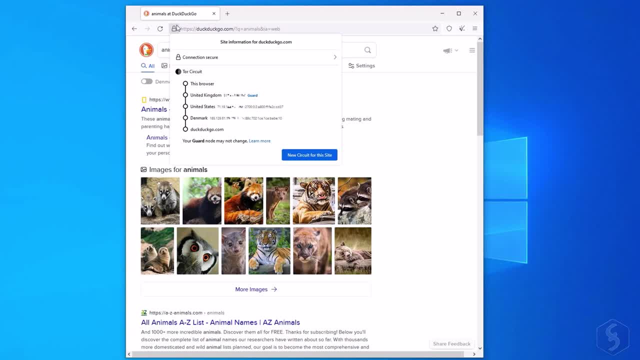 Tor Browser provides the tightest protection over your data while surfing the internet, since it blocks data tracking from websites, performs automatic cookie cleanup, hides any data you have and allows you to surf the internet. Tor Browser provides the tightest protection over your data while surfing the internet, since it blocks data tracking from websites, performs automatic cookie cleanup. 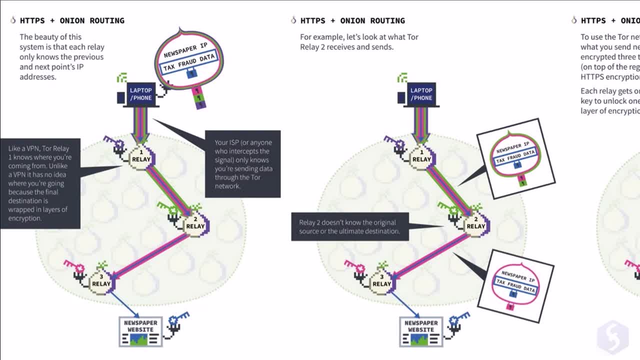 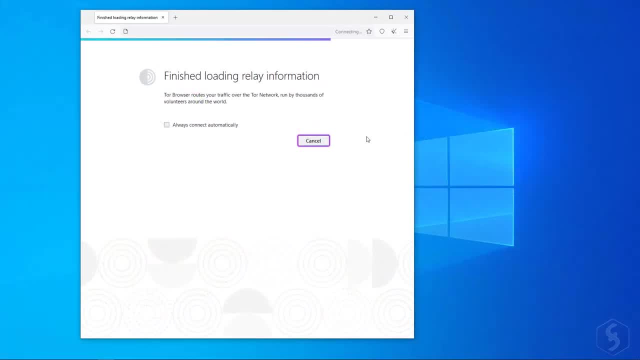 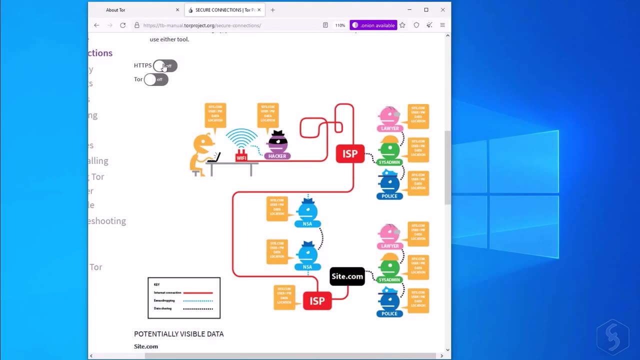 keeps internet activity from internet service providers and keeps safe your information from your devices thanks to its fingerprint protection. When you open Tor Browser, click on Connect to run and establish a secure Tor circuit. This relies on a three multi-level encryption where you connect to three relays in series before opening the destination address, just like the layers of an onion. 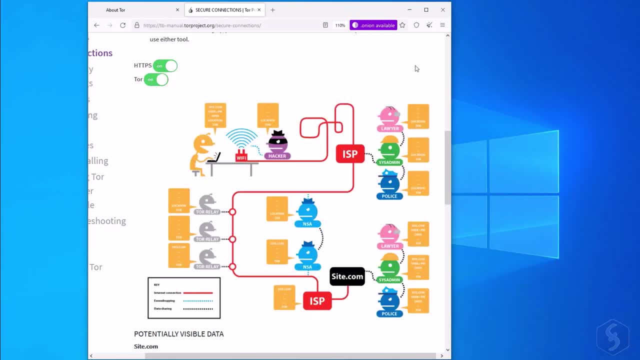 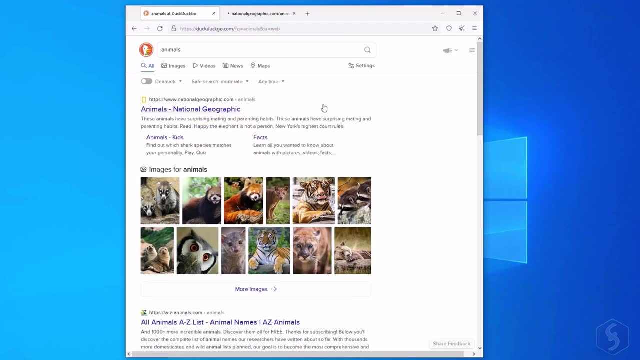 On one hand, this really keeps your data secure from other people and also gives you the possibility to visit blocked sites. On the other hand, this three-layer connection slows your line connection down, so you may not use Tor when downloading large files. 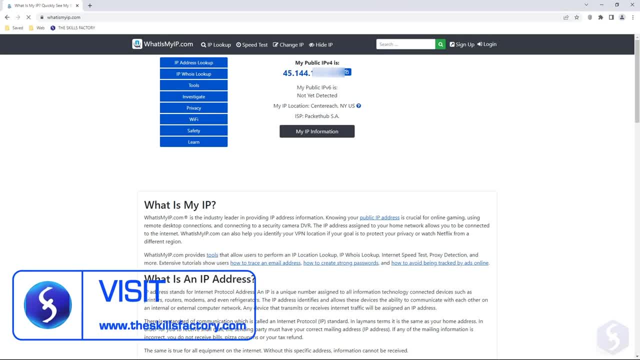 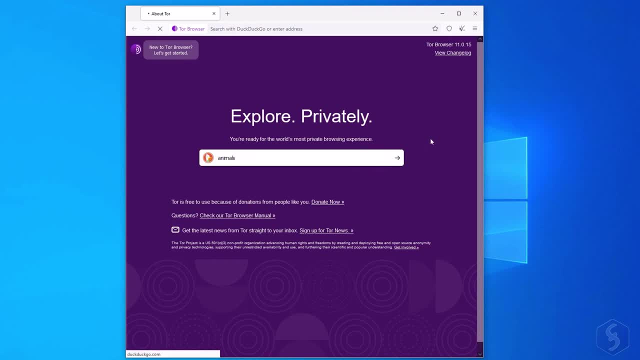 To verify this. you can make a check on your IP address or identity with a common browser and with Tor You can also search for any website with Tor. This uses DuckDuckGo as search engine, which does not save or track any personal data. 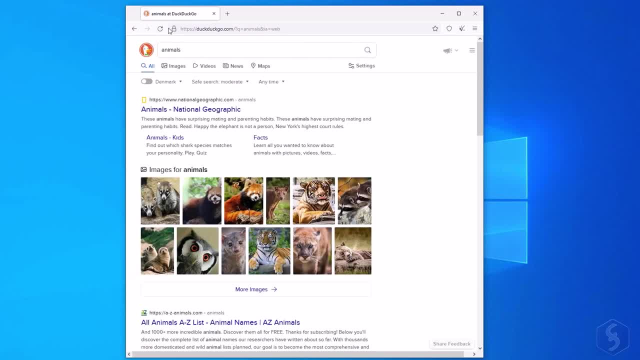 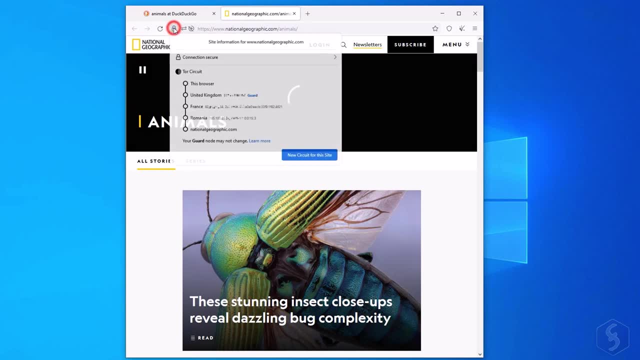 On top you get a closed lock button when the current connection is secured under the HTC. You can also check the whole Tor circuit used, including the IP addresses of the three relays, such as the guard one, the middle one and the exit one. 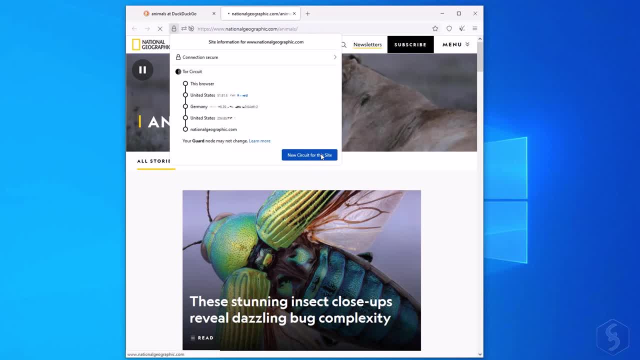 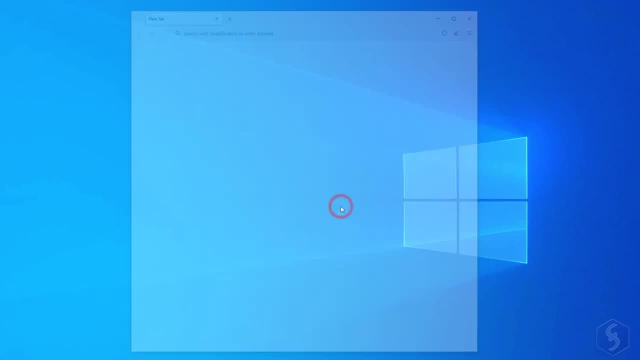 If you click on New Circuit, you establish a new Tor circuit by changing the relays' addresses. You can also go to New Identity- to make a completely new identity by restarting Tor. On the right side you find several options very similar to Mozilla Firefox. 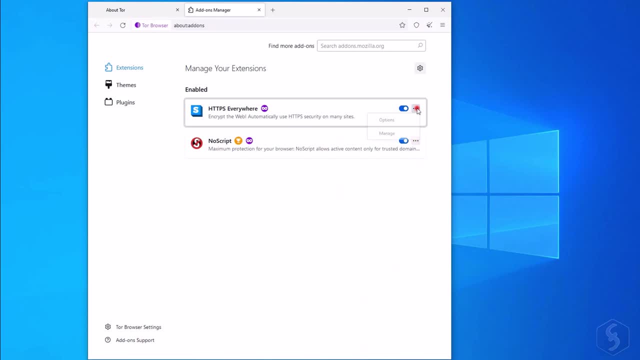 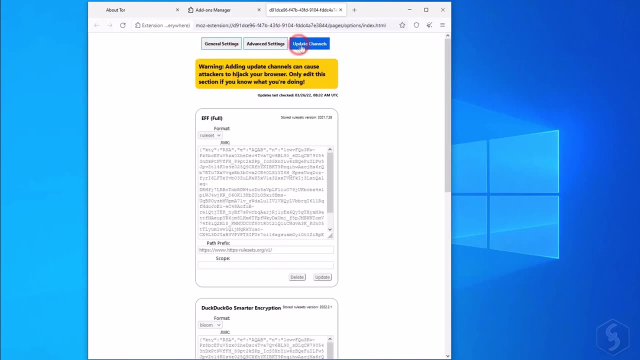 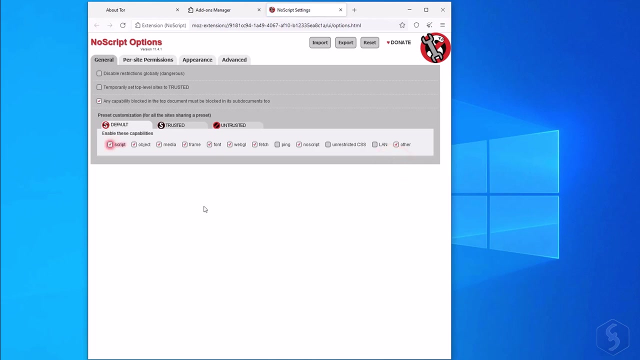 Go to Add-ons to browse, Manage and install extensions from the ones provided by Mozilla. By default. you get HTTPS Everywhere That loads just HTTPS websites And NoScript that blocks the execution of codes from non-secured sources. Besides the add-ons, you can make a new tab window identity or a new Tor circuit. 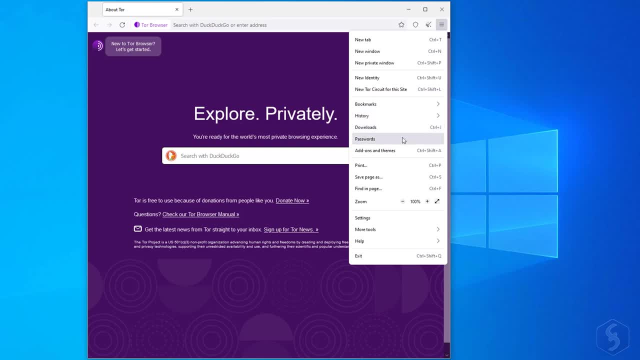 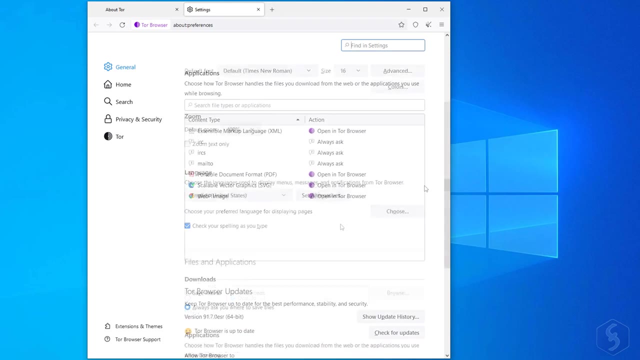 You can also save bookmarks, see your history, make a zoom on your pages, discover the integrated tools And also go to Help to find manual and additional tips. Moreover, go to Settings to change options and languages and set how to open specific file formats and manage your future updates. 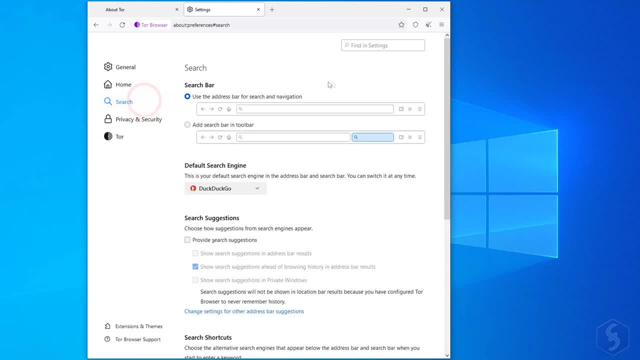 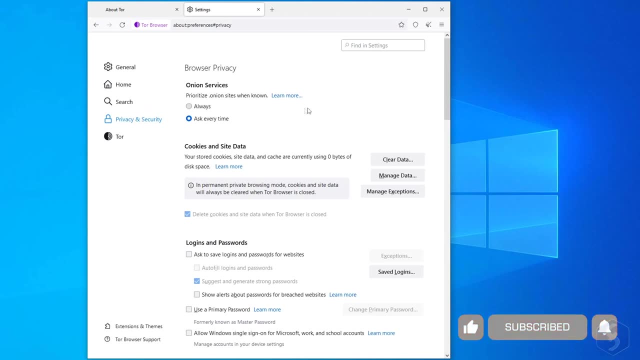 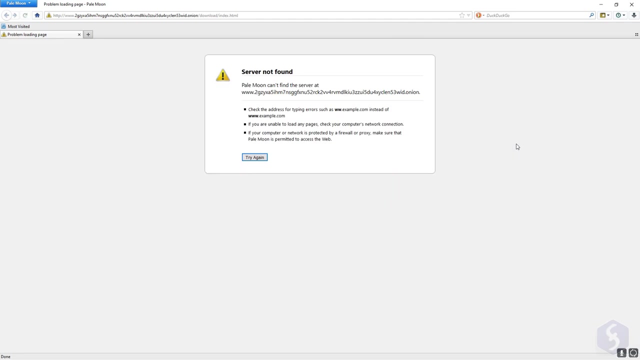 On the left, set the homepage to use the search engine and on Privacy and Security, all the options for your security. On Onion Services, you can choose to open onion websites with respect to standard domains. Onion domains can be opened with Tor only and are much safer, since they allow encryption, hide IP addresses and have no need to get a purchased domain. 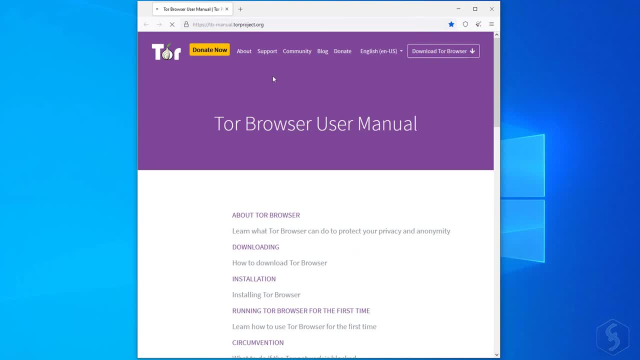 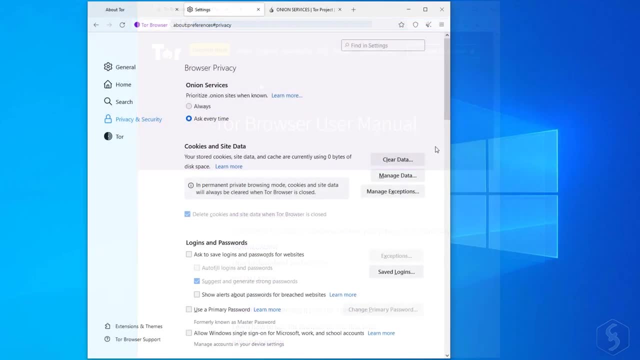 In case any website has an Onion domain, you can simply switch to the proper button on top. The Onion address is a long sequence of letters with a onion in the end. You can also clean data and manage all your saved logins and passwords. 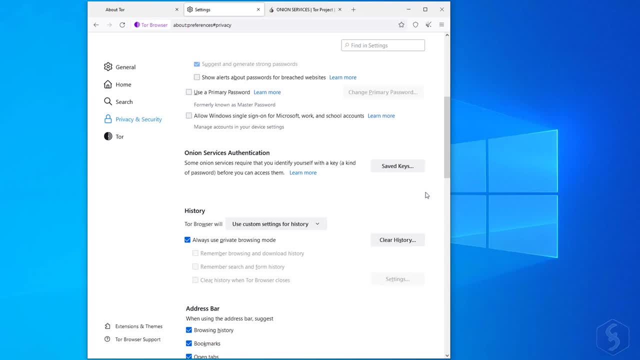 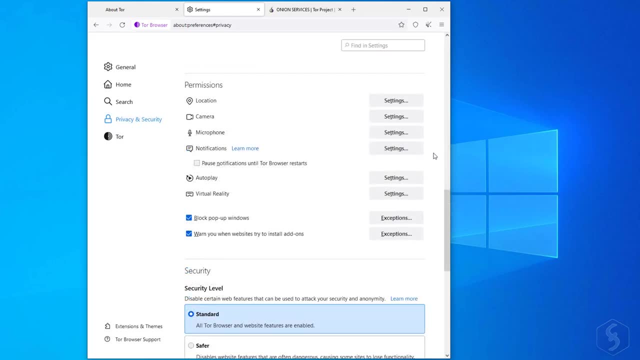 On Onion Authentication, you get the list of the saved Onion keys, Such as passwords needed to open some Onion websites for an additional level of security. On Security, set the level for the Tor browser Standard is the default option for the best user experience across most of websites. 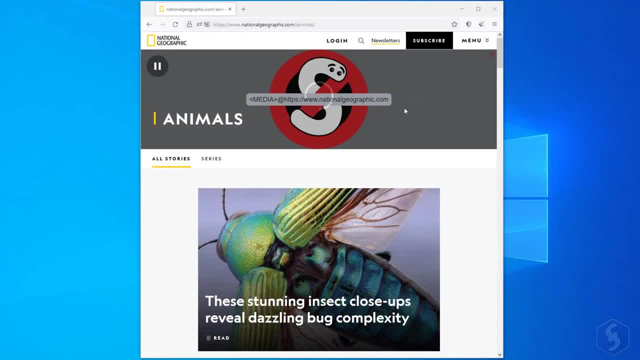 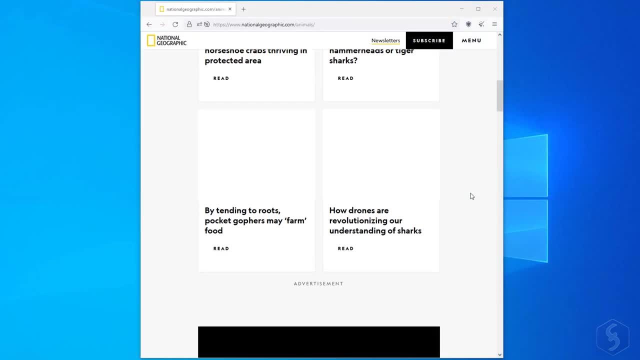 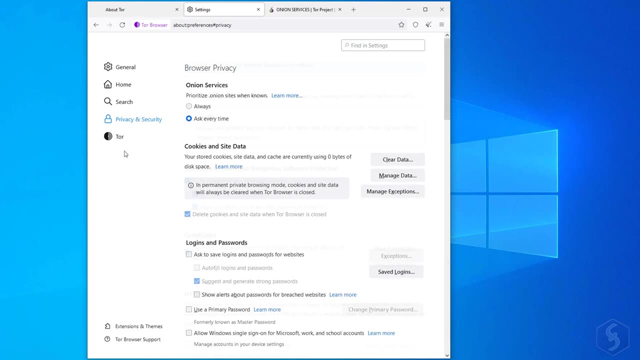 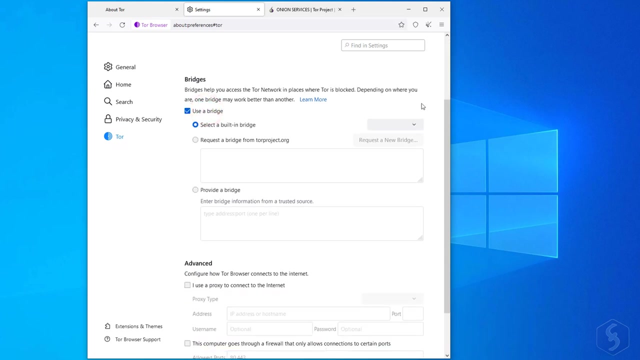 If you choose Safer, you may lose some functionalities such as playing video, Whereas use Safest to visit suspicious websites. by loading only text and a few scripts At the bottom, you can block dangerous content and downloads automatically Under Tor. you can enable the connection to the Tor network automatically or configure a bridge to be able to visit blocked websites. 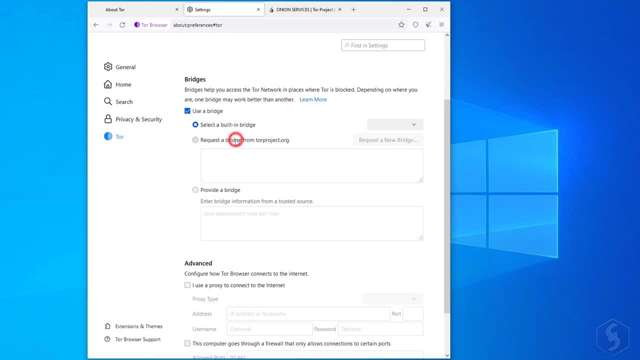 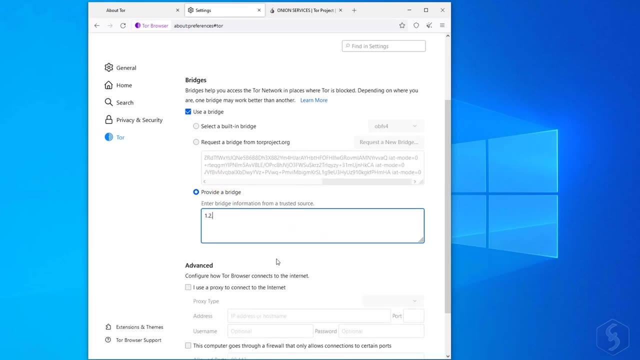 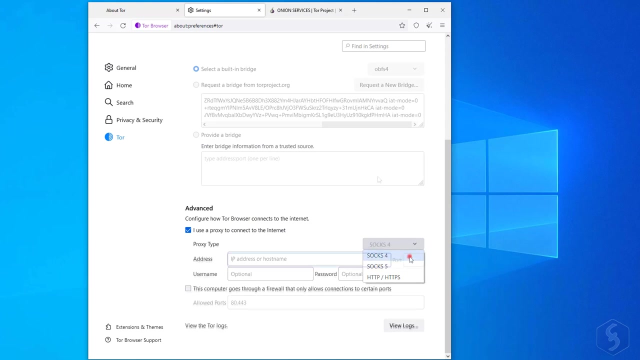 Select a built-in bridge or, in case none of the proposed ones works, you can forward a request to torprojectorg Or provide a bridge with proper IP address and port. On Advanced, you can set any proxy, specifying its type, its IP address and proper credentials.